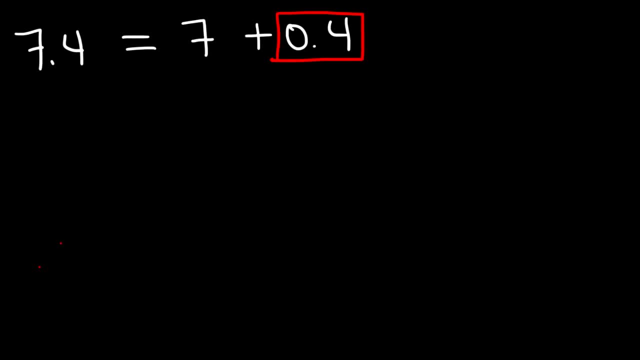 Let's focus on converting 0.4 into a fraction, So 0.4 is a decimal that stops at the tenths place, just like the last problem. So we're going to multiply the top and the bottom by 10.. 0.4 times 10 is 4.. 1 times 10 is 10.. 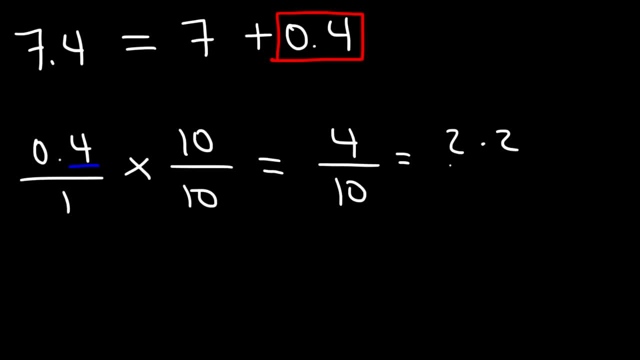 So we have 4 over 10.. 4 is 2 times 2.. 10 is 2 times 5., And so these will be cancelled, And so this is 2 over 5.. So 0.4 is equal to 2 over 5.. 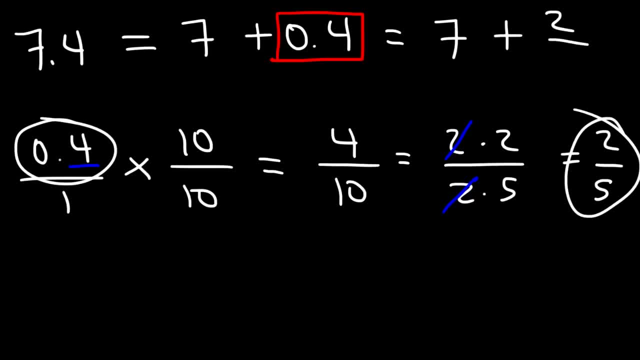 So we have 7. Plus 2 over 5, which is the same as 7 and 2 fifths. So 7.4 is equal to 7 and 2 fifths as a mixed number. Now what if we have a decimal that's rounded to the hundredths place? 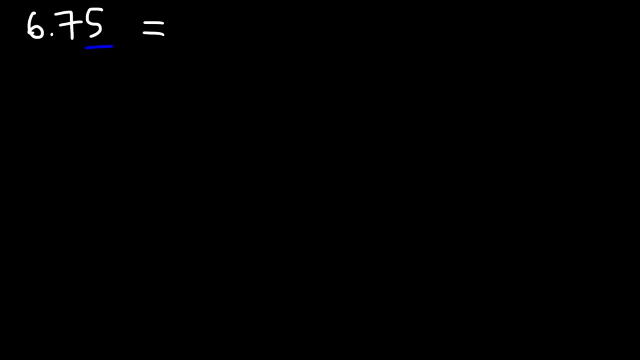 What do we do in this case? So feel free to take a minute and work on this example, Pause the video if you have to And try this problem. So first I'm going to separate the whole number from the decimal portion of the number. 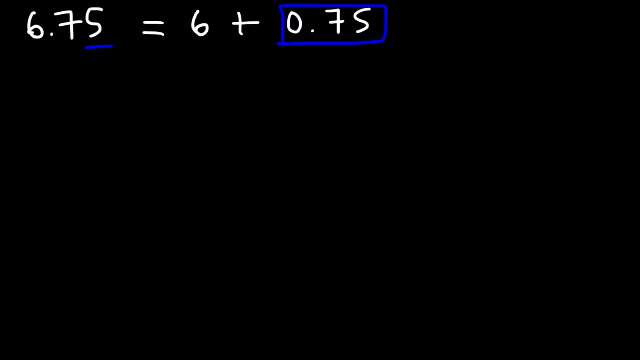 And now let's convert 0.75 into a fraction. So because 0.75 is at the hundredths place, I'm going to multiply the top and the bottom by 100.. 0.75 times 100 is 75.. 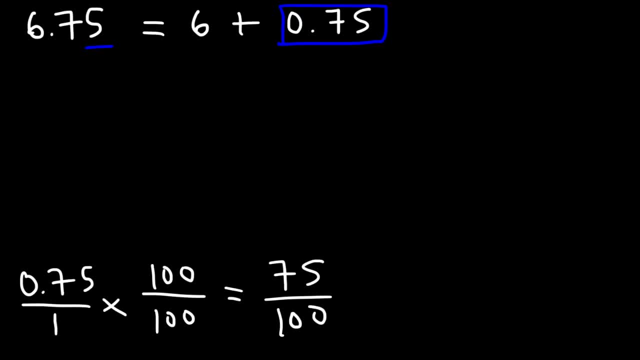 And 1 times 100 is 100.. So if you look at the last digit, if it's in the hundredths place, multiply the top and the bottom by 100.. If it's in the thousandths place, multiply the top and bottom by 1000. 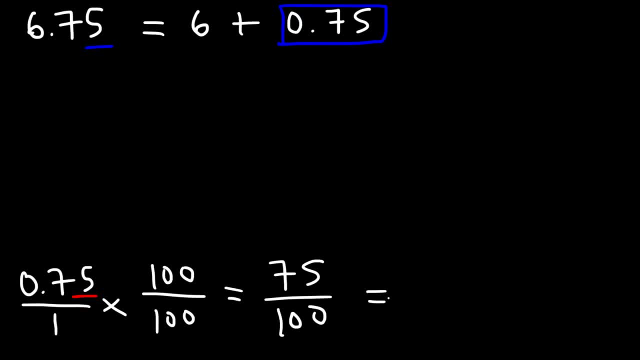 Now we need to simplify: 75 over 100.. 75 is 25 times 3.. 100 is 25 times 4.. So we can cancel a 25.. And this is going to give us 3 over 4.. So 0.75 is 3. fourths, 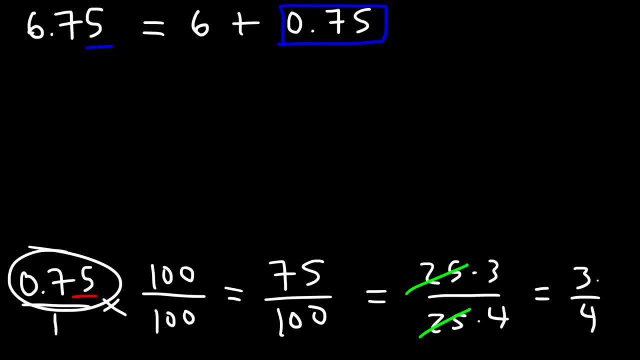 So this becomes 6 plus 3 over 4.. And this is going to give us 3 over 4.. So 0.75 is 3 fourths. So this becomes 6 plus 3 over 4. Which is 6 and 3 fourths. 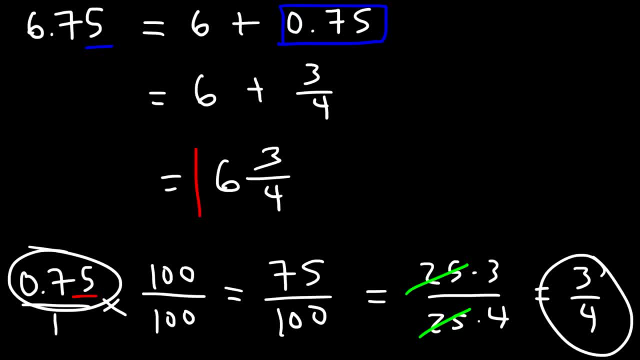 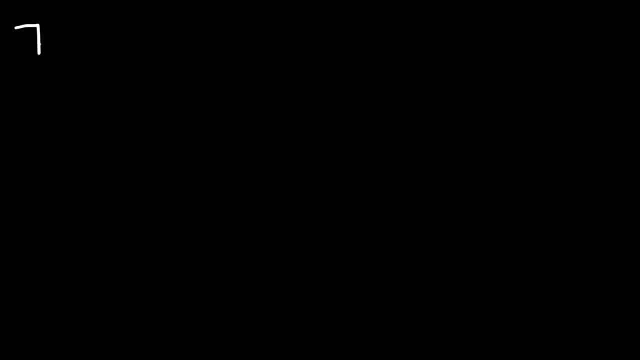 So that's how you can convert that decimal into a mixed number. Now, what about this one? 7.625. So notice that the last digit is in the thousandths place, So keep that in mind. So let's write this as 7 plus 0.625. 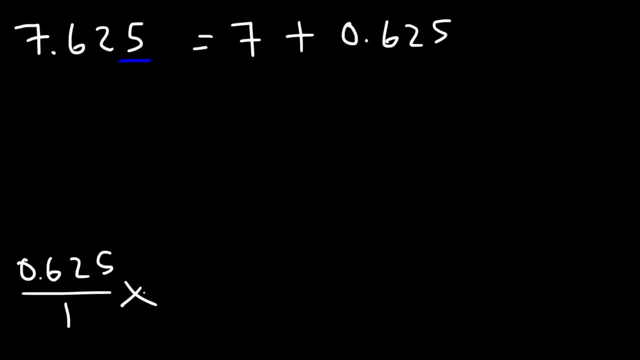 So, because the last digit is in the thousands place, we're going to multiply the top and the bottom by 1000.. 0.625 is 625, and 1 times 1000 is 1000.. Now what is the best way in which we could simplify this process? 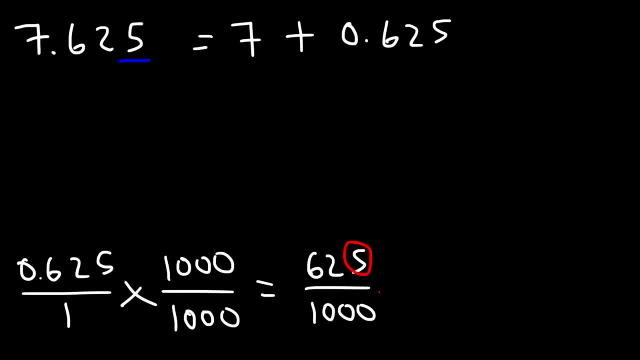 So notice that the last two numbers, I mean the last number of 625, is a 5, and for 1000 it's a 0. If a number ends in a 5 or a 0, you know it's divisible by 5.. 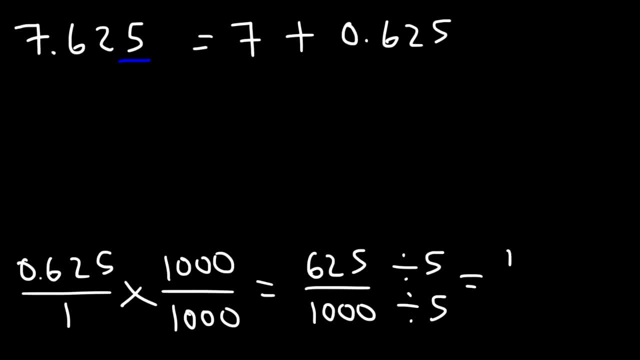 So 625 divided by 5 is 125, and 1000 divided by 5 is 200.. So we have 125 over 200.. Now how many quarters is equal to $1.25? It takes 5 quarters to have 25.. 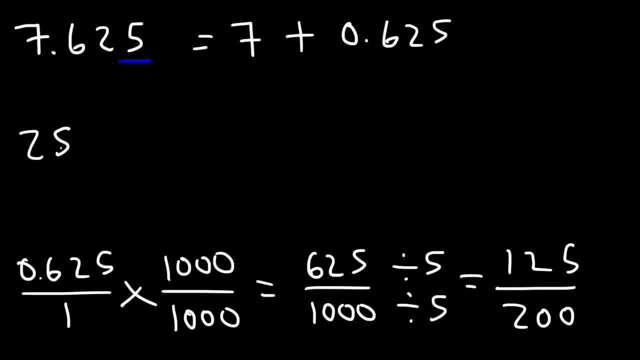 So 125 is basically 25 times 5.. And how many quarters do you need to make $2? You need 8 quarters to make $2. So 200 is 25 times 8.. You know what, when you think of money, math makes sense. 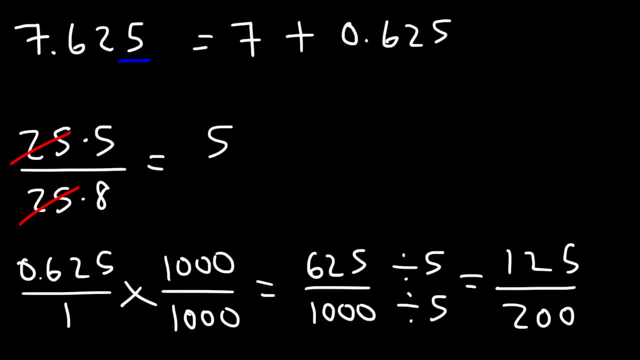 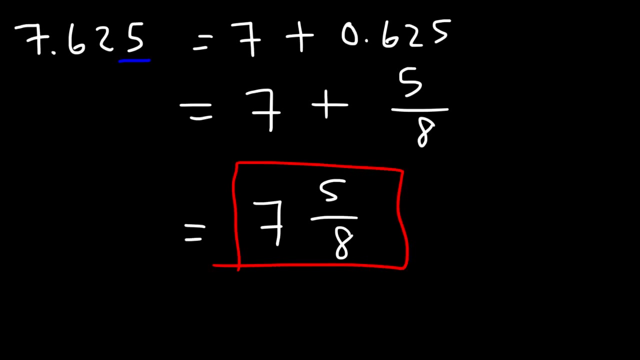 So we could cancel 25.. And so 5 over 8 is equal to 0.625.. So let's replace 0.625 with 5 over 8.. So our final answer is 7 and 5 eighths. 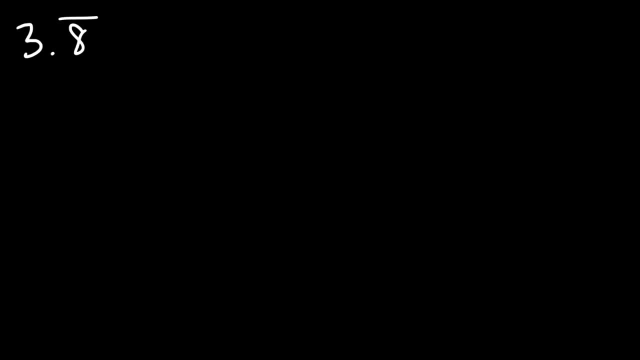 Now let's try this one: 3.8 repeated. What is the answer? How can we convert that into a mixed number So we can express this as 3 plus 8.. So we can express this as 3 plus 8.. 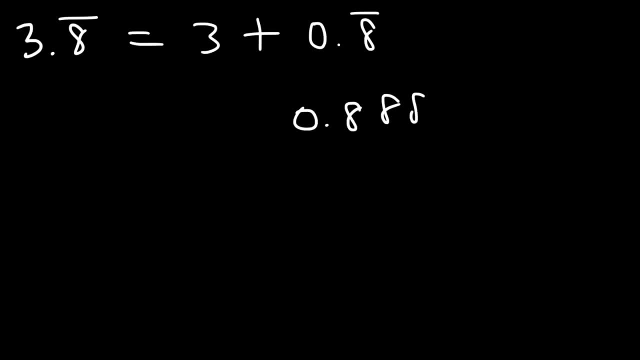 0.8 repeated. 0.8 repeated is 0.88888, and that just goes on forever. So what do we need to do when dealing with a repeating decimal Point, 2 repeating, for example? you just need to know that it's 2 over 9.. 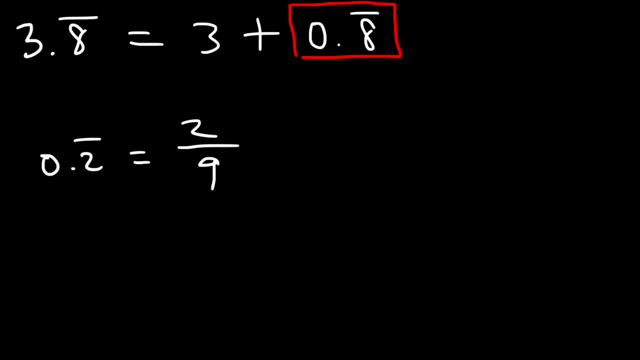 If you take your calculator and if you type in 2 divided by 9, you're going to get point 2 repeating. If you type in, let's say, 4 over 9, you'll get 0.4 repeating. 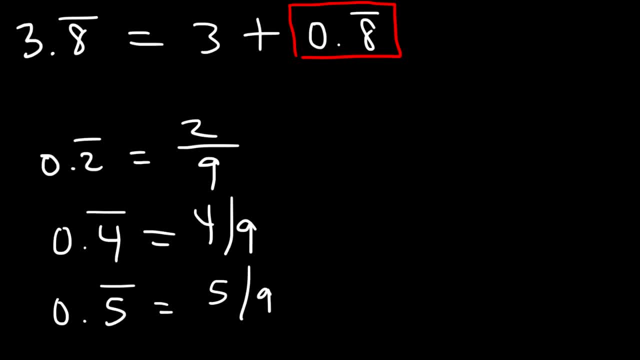 0.5 repeating is simply 5 over 9.. And these are some things you just need to know. So, therefore, 0.8 repeating is simply 8 over 9.. So the final answer is 3 and 8 over 9.. 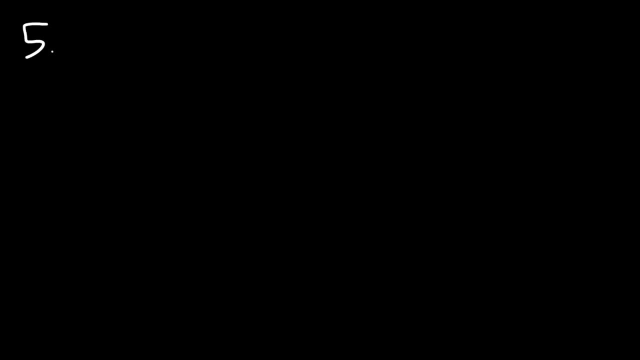 So if that's the case, what about this one? 5.23 repeated. So that's going to be 5 plus 0.23 repeating. And what do you think 0.23 repeating is equal to? For example, 0.34 repeating is 34 over 99.. 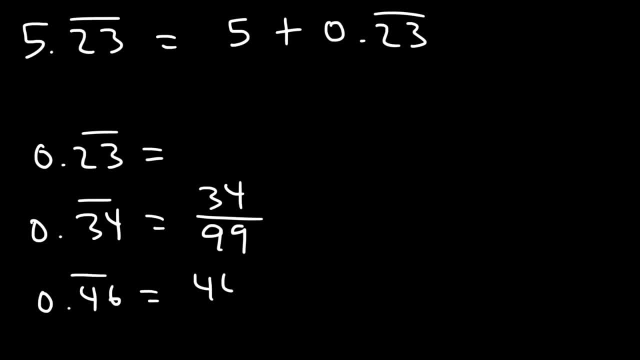 0.46 repeating is 46 over 99. So you just got to add another 9, because you have 2 numbers that are repeated as opposed to 1. So 0.23 is 23 over 99. So that's going to be 5 plus 0.23 repeating. 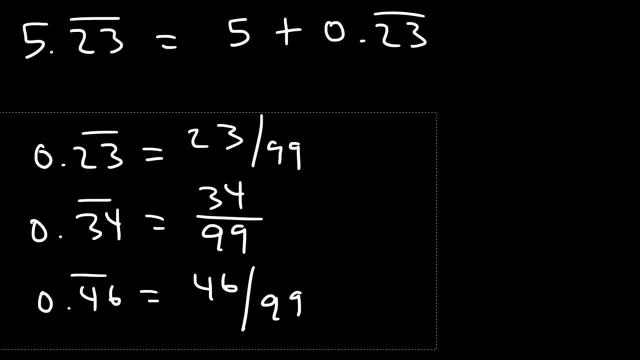 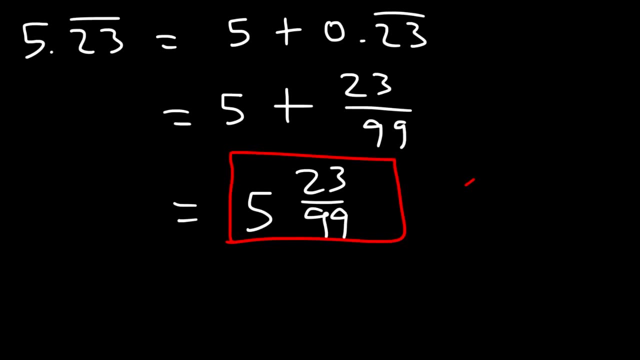 That is 0.23 repeating. So this becomes 5 plus 23 over 99. And so the final answer is 5 and 23 over 99. So that's 5.23 repeating. So here is a challenge problem for you. 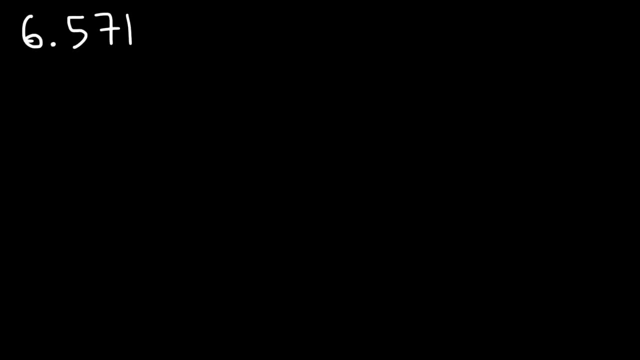 Let's say, if we have the decimal 6.57171717.. Okay, And it keeps on following that pattern. How can we convert that decimal into a mixed number? So first I'm going to write this as 6 plus 0.571717171. 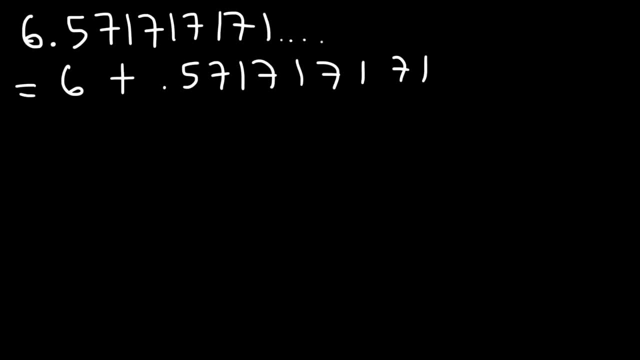 Now we need to identify what's repeating and what's not repeating. So we know that the 0.5 is not repeating, But we can see that, Okay, The 7 and the 1, that's repeating. So what is the repeating element? 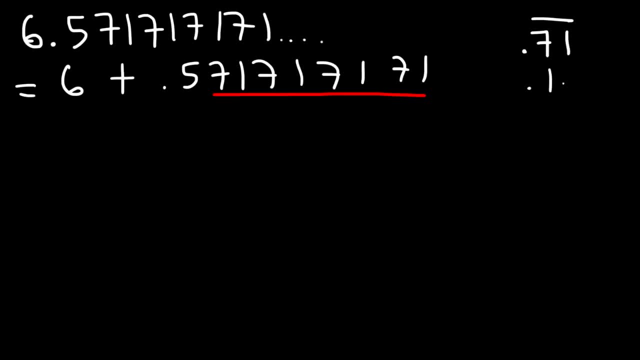 Is it 0.71 or is it 0.17? That's what we need to determine Now. it doesn't make sense that it's 0.71, because 0.71 is greater than 0.5.. So we're going to try 0.17.. 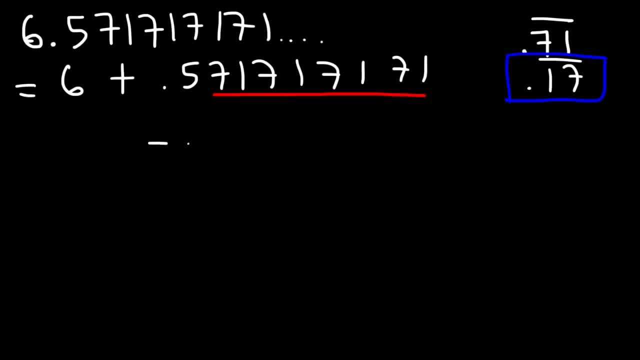 So if we take this number and subtract it By 0.17, repeating What's going to happen. So notice that this portion will completely cancel. So we get 0.57 minus 0.17, which is 0.4.. 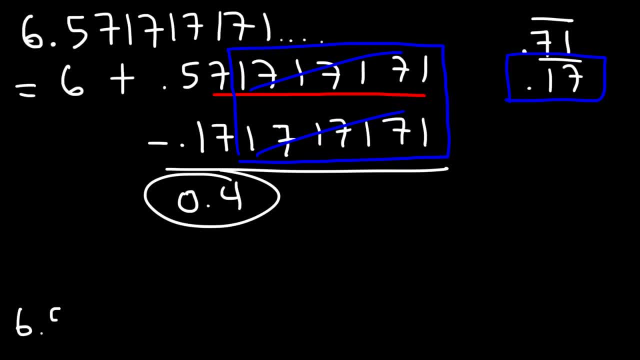 So we get a fixed value. Therefore we can say that 6.571717171. Is basically 6 plus 0.4 plus 0.17. repeating That will give us our original number. So now that we broke it down, 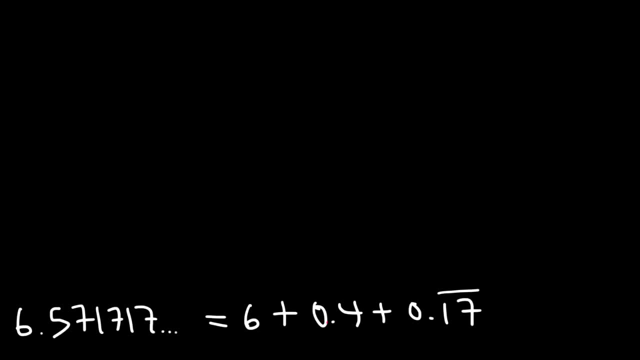 We can focus on converting these two into fractions. So let's start with 0.4.. Okay, So let's multiply it by 10 over 10.. So this becomes 4 over 10.. And if we divide both numbers by 2.. 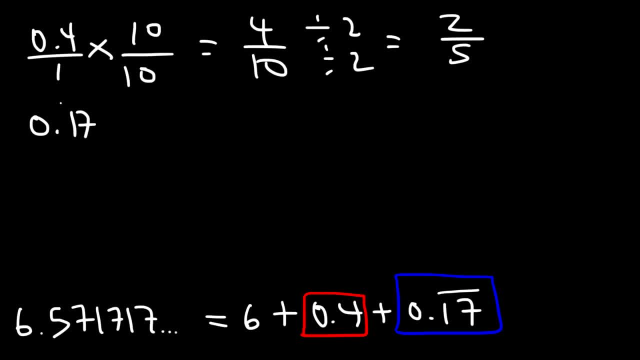 We'll get 2 over 5.. And we know that 0.17 repeating Is 17 over 99. So therefore We can say that this number- 6.571717. Is really 6 plus 2 over 5.. 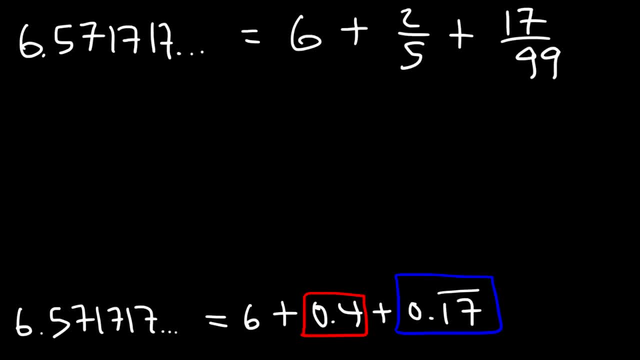 Which equals 17 over 99.. The last thing we need to do Is convert these two fractions into a single fraction, So we need to get common denominators, Or we could use a simple technique. We can multiply 5. And 99..